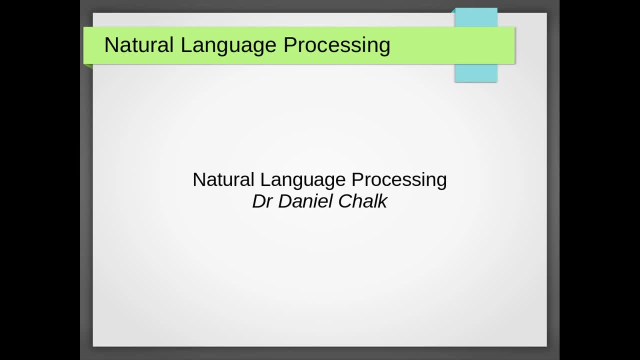 actual code writing. We're going to be talking mainly about the processes and about some of the theory behind natural language processing, more than actually how you do this yourself, But I will be showing you links of areas where you can look for further information on some of 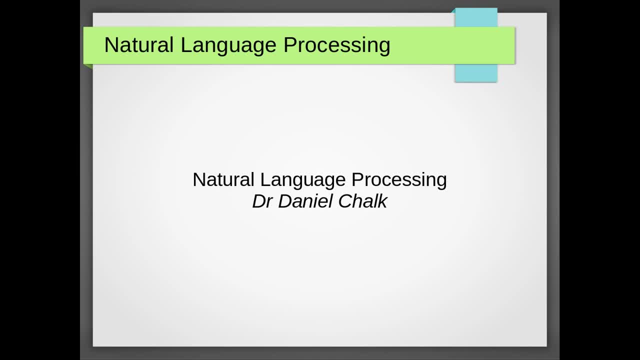 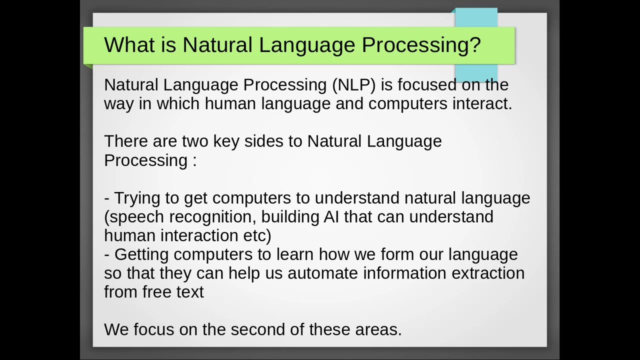 this stuff and also showing you a little bit more of a worked example using a piece of software called spaCy, which we'll be taking you through in a little while. So what do we mean by natural language processing? Well, natural language processing, which is commonly abbreviated to NLP, is focused on the way in which computers interact with human 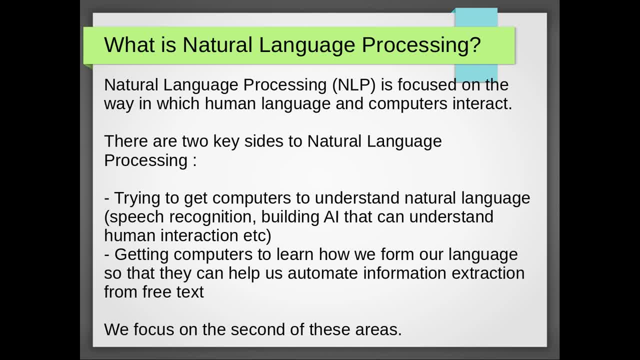 language And there are two kind of key areas to natural language processing. There's the side in which we're trying to get computers to understand natural language in some way, That we're building an AI to try to get our computer to understand what we're saying to it. So that covers. 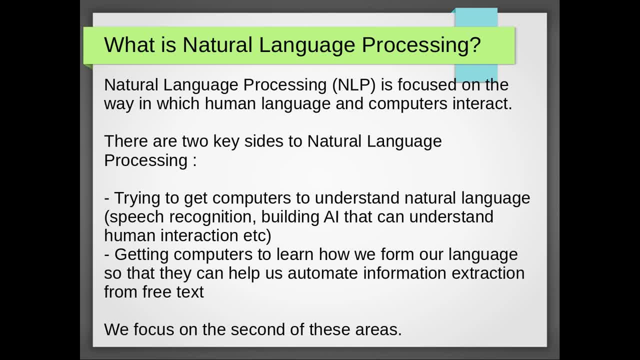 speech recognition, kind of automated bots etc. that you see online, where they're trying to understand what somebody has said, when they're, when they're trying to communicate to them. And then there's the other side, which is the area that we're more interested in, which is actually 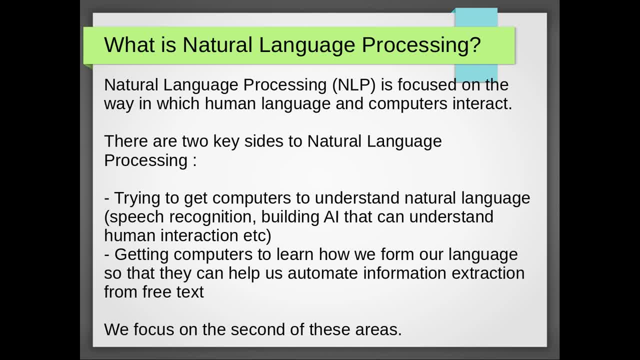 getting computers to learn how we form our language in order that they can help us to understand our learning, so that we can start to get it in some way. We know that some ThreeD functions will be more powerful in a few years time, so that we can start to get it together. 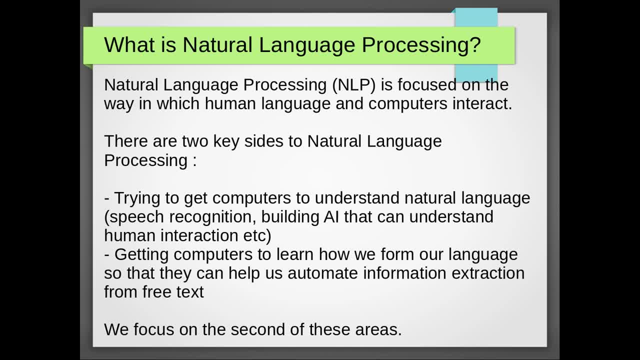 So let's talk a bit more about what we do. so we're going to be looking at a larger range of training, and this is an opportunity to get into the data base- not just device types, but even data sources, So we often need to be familiar with a few of them. So when I first started working with 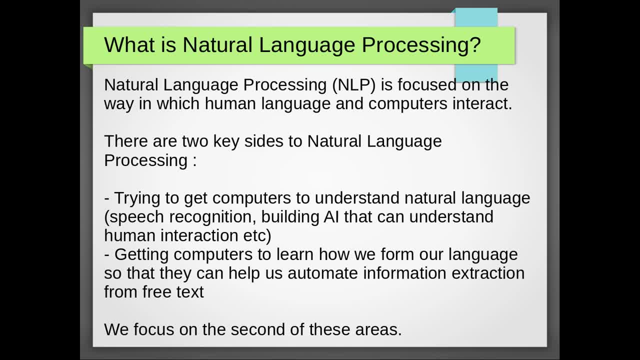 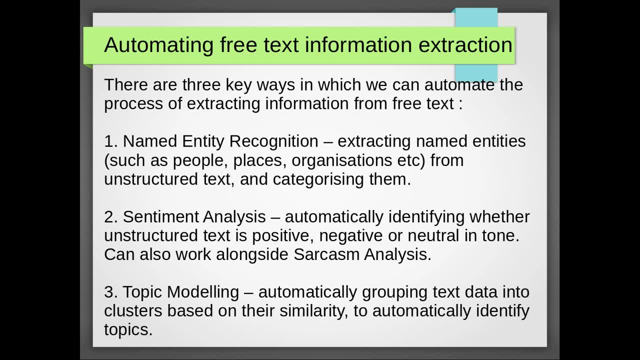 so that's the side that we're going to be focusing on today and in terms of that area of automating free text information extraction, there are kind of three main areas in which we can automate the process of extracting information from free text. the first one is something called named entity. 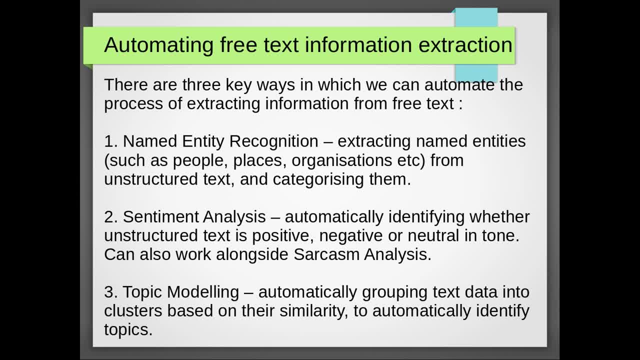 recognition. named entity recognition is where we try to extract what are known as named entities. these are things like people, places, organizations, countries, those sort of things- from free text and categorizing them, and we'll come on to in a moment why that might be really useful. the second area is 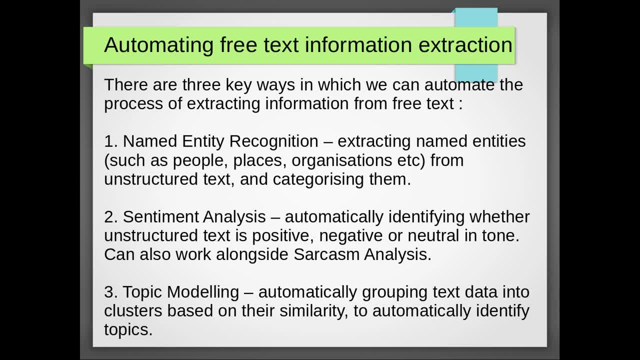 something called sentiment analysis. sentiment analysis is all about trying to identify whether some free text is either positive, negative or negative, maybe neutral in tone, and there's also something that goes hand in hand with that called sarcasm analysis, which we'll come on to later, and again this can be really useful for trying to extract. 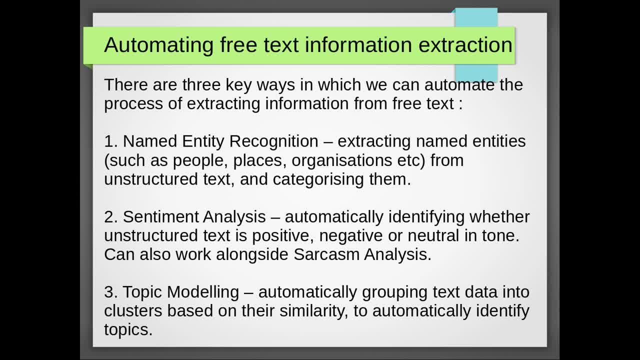 information in a different way from free text. and the third area is something known as topic modeling, and in topic modeling what we're trying to do is to automatically group texts into clusters based on these text classes, so we're automatically kind of grouping things into similar topic areas. 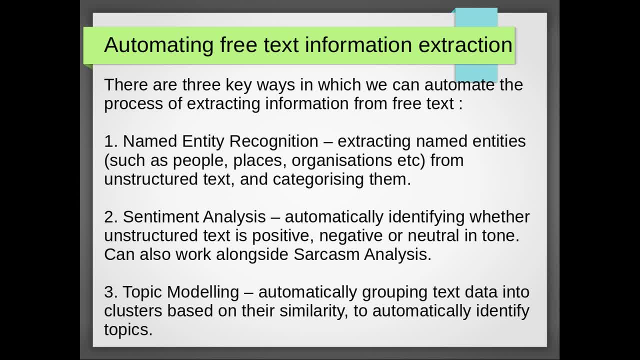 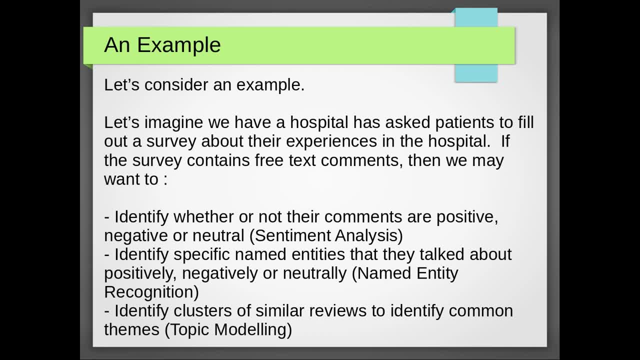 and we're not going to go into topic modeling today, but i will at the end show you where you can go and read a little bit more about that. so that will sound sort of very theoretical at the moment. so let's ground this with an example. so let's imagine that we've got a hospital and the hospital has asked patients to fill out a survey. 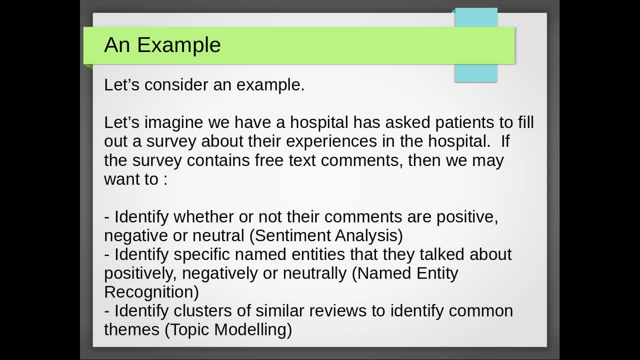 based on their experiences in the hospital survey contains free text comments, which very often they will. then what we may want to do is we might want to look to see whether the comments are positive, negative or neutral. So we want to apply some sort of sentiment analysis to this. 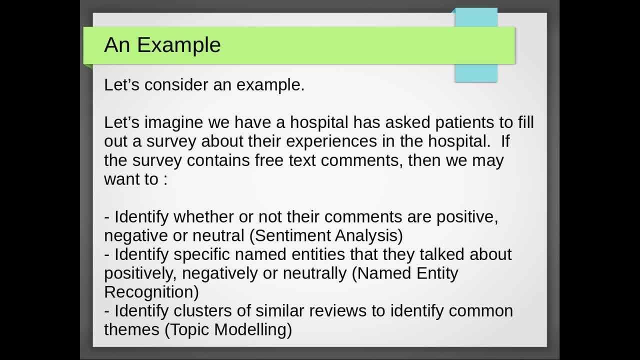 We may want to look for specific named entities that are being talked about positively, negatively or neutrally, which is the named entity recognition side. So we may not just want to know whether this review was positive, but also to say what were the things that were being talked about in our positive 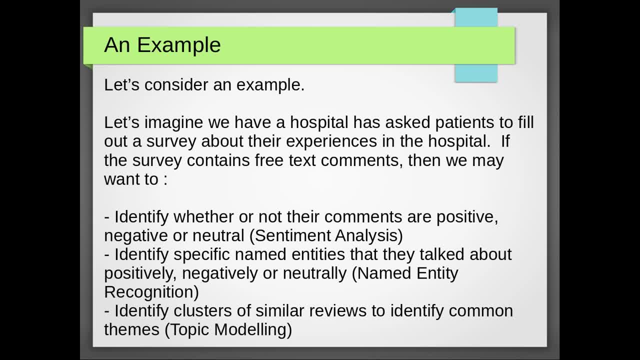 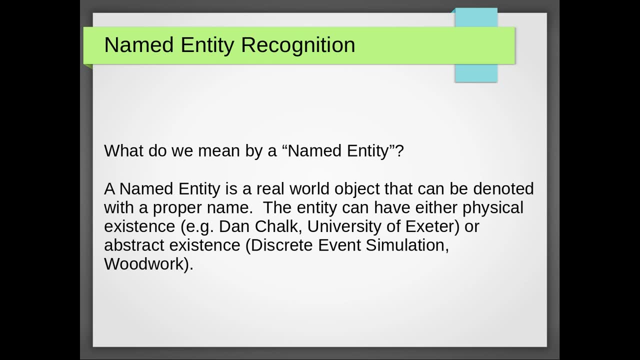 reviews versus our negative reviews, for example. We may also want to identify clusters of similar reviews to try and identify common themes, and that's where topic modeling might come into play. So let's start with named entity recognition. So what do we mean by a named entity? So a named entity is a real 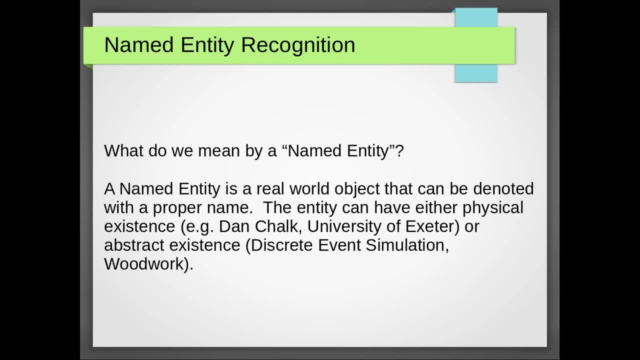 world object that can be denoted with a proper name. So a named entity can either have a physical existence- for example Dan Chalk University of Exeter, These are both things that exist- at least I hope I exist- or they may have a more abstract existence. so concepts like 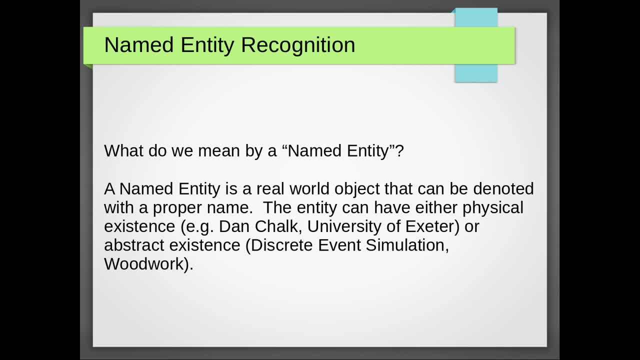 discrete event simulation that's not a physical thing, but it is a named entity. Woodwork cookery: These are examples of abstract existence, According to alama at r, the University of Exeter. resistances, but they are still named entities and the sort of things that we would want to. 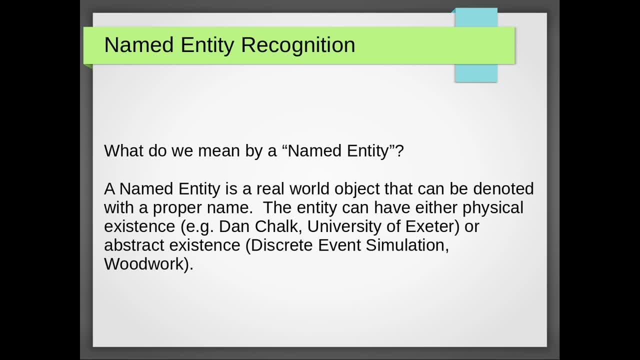 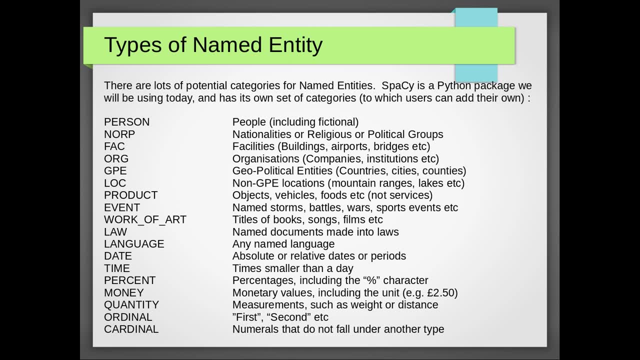 try and extract when we're undertaking named entity recognition And, as it turns out, there are lots of different potential categories for named entities And I'm putting this up here from so that there are lots of different sort of category lists depending on the package that 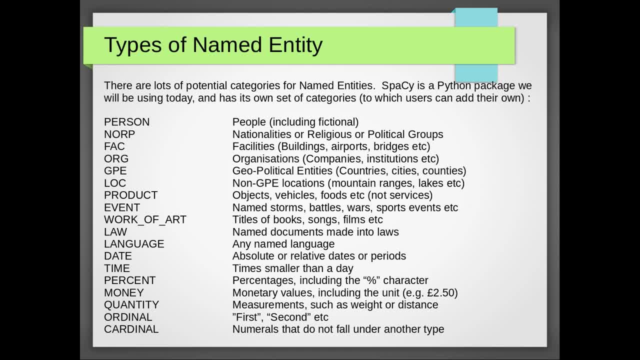 you use. spaCy is a Python package that we're going to be using today and is probably one of the most widely used, if not the most widely used- natural language processing parsing package today, And spaCy has its own set of categories. This isn't a finite list. These are: 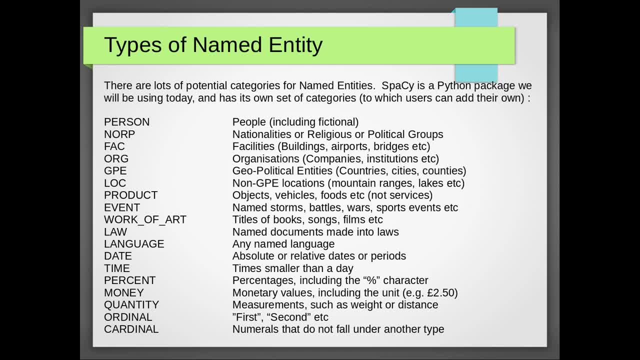 the sort of default categories, but users can add their own categories to this as well. So in spaCy there are a number of categories that we're going to be using today, And I'm going to go through them one by one. So in spaCy you've got the idea that named entities can be of type. 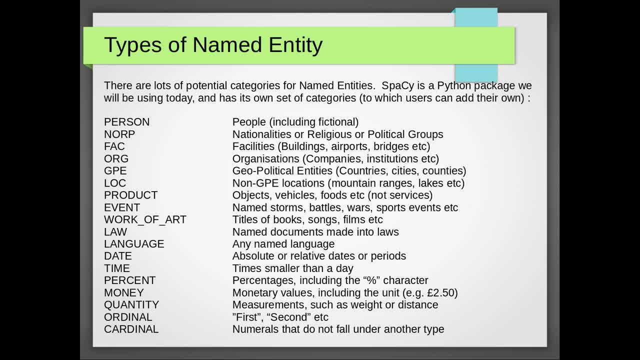 person. Person basically just means that these are people, and that can include fictional people, fictional characters as well. It can be NORP, The category NORP stands for nationalities or religious or political groups. We can have FAC, which stands for facilities. These are things. 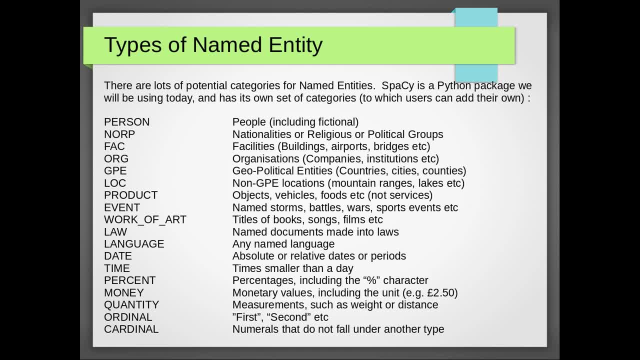 like buildings, airports, bridges, et cetera. These are all named entities. There's a category called org, which you've probably guessed stands for organizations. These are things like companies, institutions, et cetera. There's a category called GPE. These stands for geopolitical. 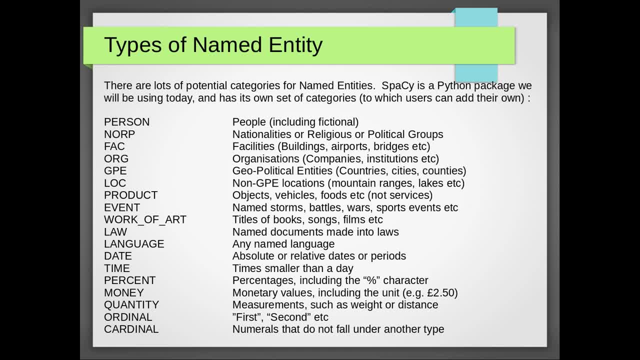 entities. So these are things like countries, cities, counties, these geographical and or political structures, LOC, which stands for non-geopolitical entity locations, So things that wouldn't fit into GPE but which are locations on the left. So think of things like mountain. 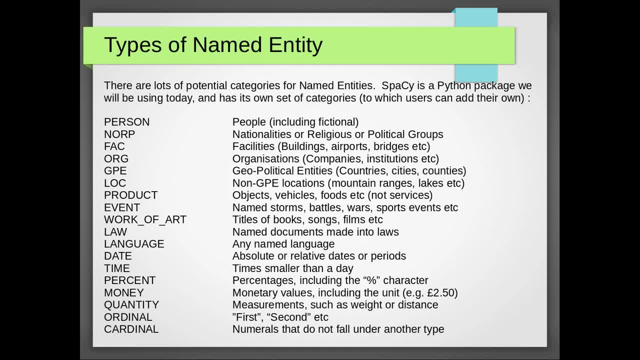 ranges or lakes, et cetera. They wouldn't come under GPE, but they would come under the LOC category. We've also got a category called product. This captures things like objects, vehicles, foods, et cetera, but not services. We've got a category for events, So think of things like. 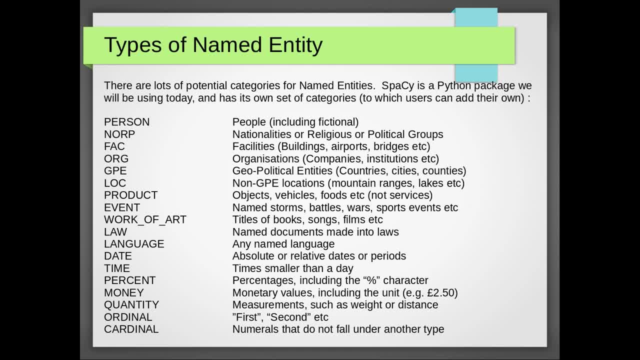 name storms, Battles, wars, sporting events et cetera. Works of art, So that captures things like titles of books, songs, films, those sort of things. Law, that's for name documents that have been made into laws. Language which represents any name language: English, French, et cetera. Date Now: 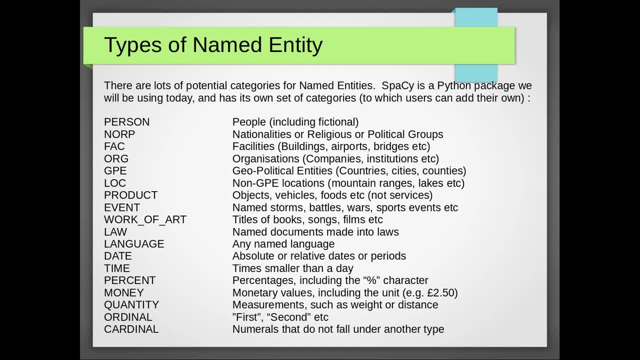 this is an odd one that you may. as you go down this list, you might be surprised that some of these things are named entities, but they are very much named entities. So dates, which in named entity recognition terms, we mean absolute or relative dates or periods. So 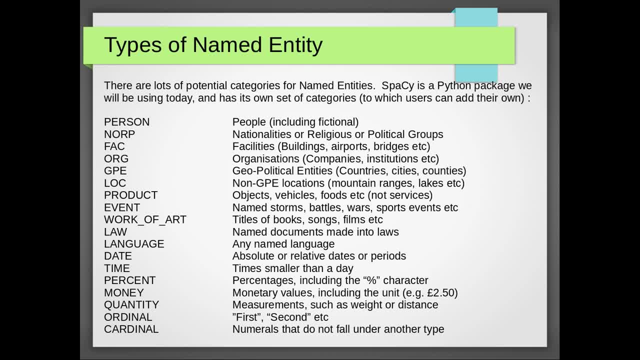 it might be something like the 1st of January 1962, or it might be something like last month. Last month would also be a named entity of type date. We've also got the concept of time. So times are named entities and time- the time category here, captures any named entities that are times which. 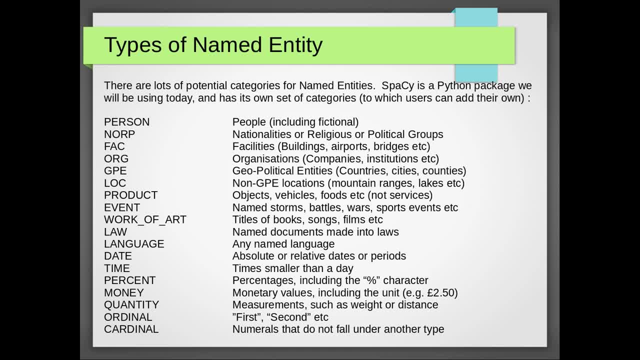 are smaller than a day, So 12 minutes to two, three hours ago. Percent. So this captures percentages and they are represented as named entities And, for the avoidance of doubt, the named entity, if it's a percentage, will include the percentage character. 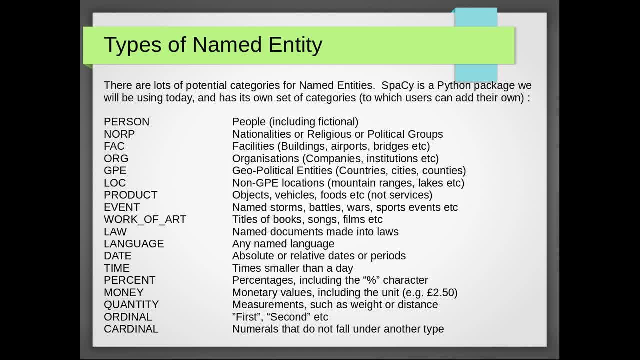 Money, So that's monetary values including the unit. so two pounds 50 would be an example of a money named entity. We've got quantity, So these are measurements such as weight or distance or some sort of quantity of something. Ordinal category named entities. 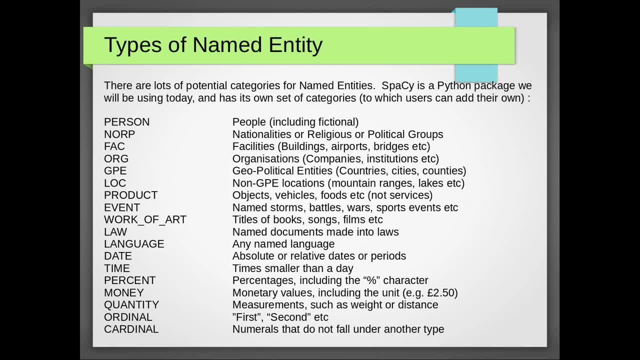 These are things like first, second, et cetera, and cardinal named entities And those are basically numbers that don't fall into one of those categories. So these are actually numbers that are actually those other types listed above: date, time, percent, money, quantity or ordinal, So any 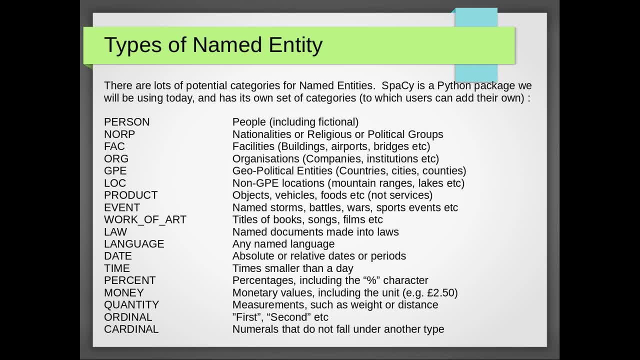 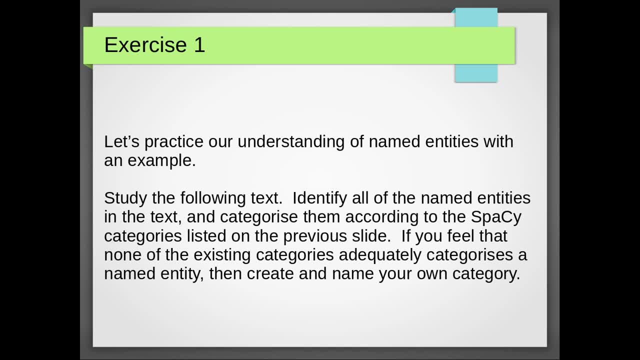 other numbers that don't fit into those categories would be classed as cardinal. So that was a whistle-stop tour of some of the basics of named entity recognition, classification and what a named entity is. So let's practice with an exercise. So just to kick things off. 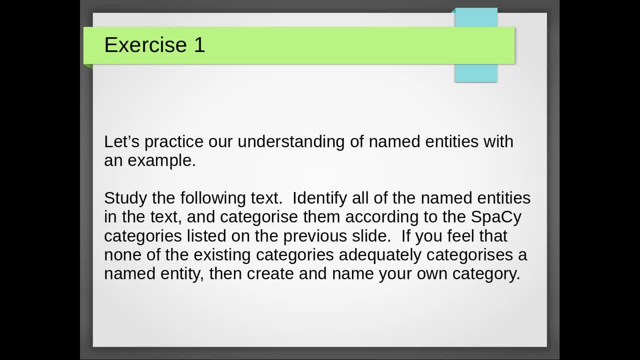 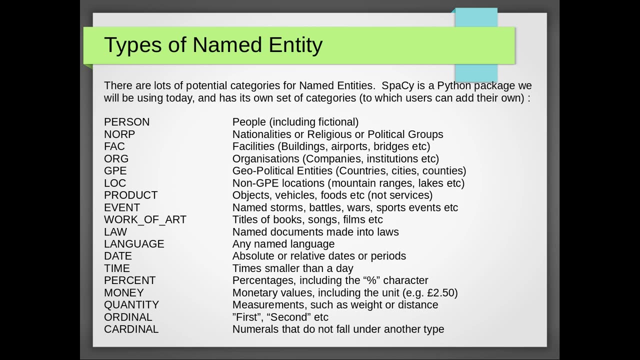 I want you to study the following text, which I'm going to throw up in a moment. I want you to identify all of the named entities in that text and I want you to categorize them according to the spacey categories that we've just talked through on this slide here, If you feel for any. 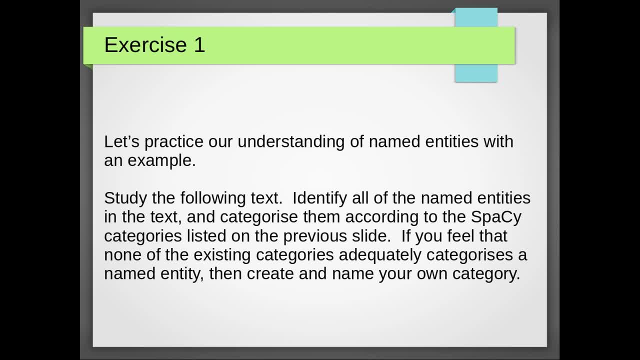 of them that they don't fit into an existing category, then either put them into the category you think they should best fit into, or either put them into the category you think they should best fit into, or if you think they really don't fit into any of them, then feel free to create and. 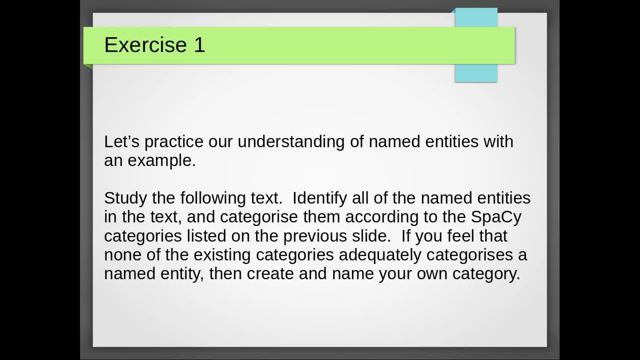 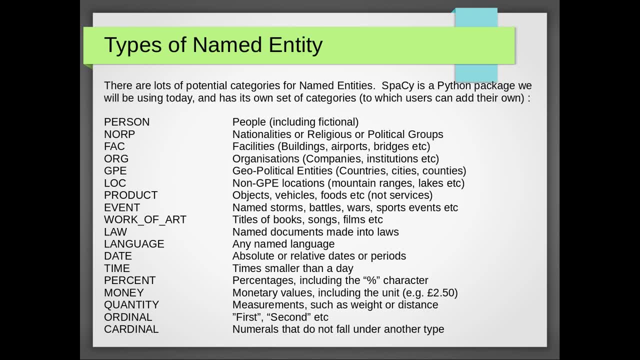 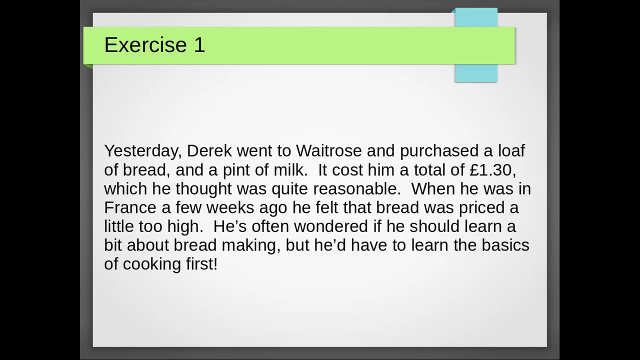 name your own category. Okay, so you're going to find all the named entities and then say what category they belong to, based on this list of spacey named entity categories. So here's your text. I'm just going to read it to you. Yesterday, Derek went to Waitrose and purchased a loaf of.